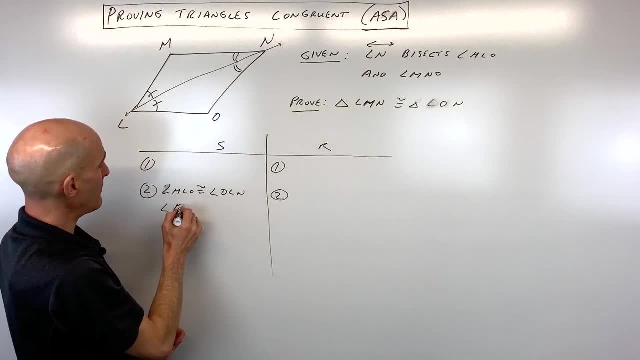 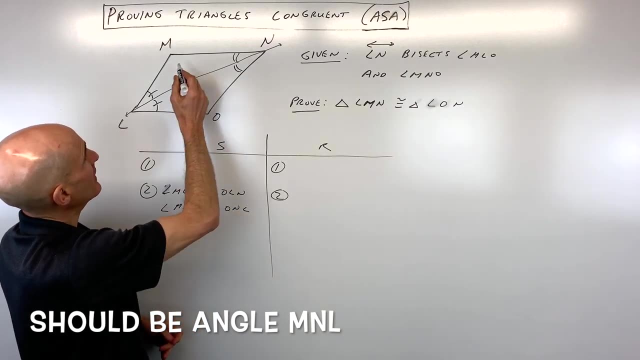 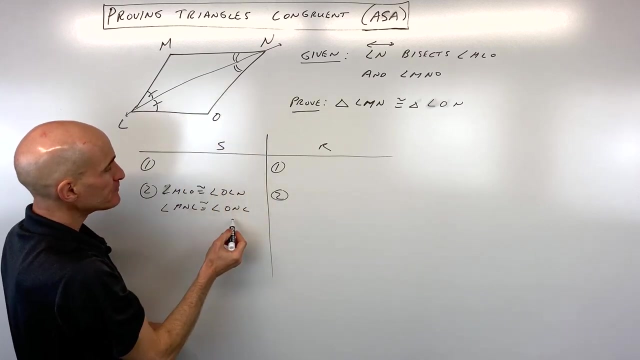 going to combine that with step number two here. This is going to be: angle MNO is congruent to angle ONL. Okay, MN, Did I say that right? MNL, sorry, angle MNL. MNL is congruent to ONL And the reason is definition of angle bisector. I'm just 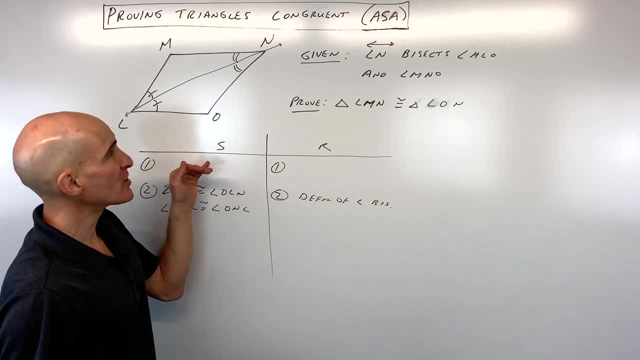 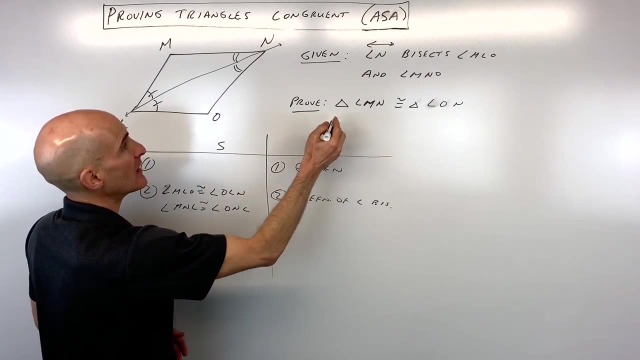 abbreviating. Now notice I skipped step number one. Step number one generally. what students like to do- and I like to do this too- is just to put your givens first. So I'm just going to write for step number one given and I'm just going to draw a line here. Okay, but you would 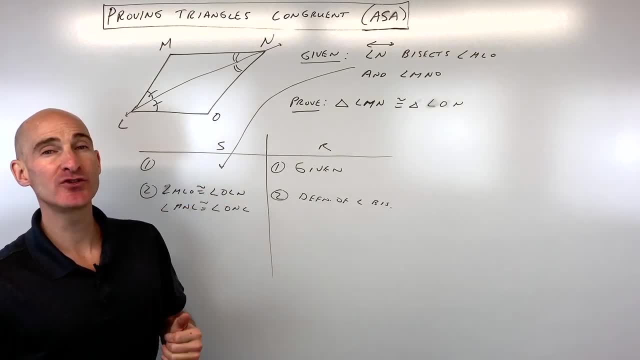 put those givens first. Now sometimes students like to put it as they need those particular givens later on in the proof so that it flows. So I'm going to put that in there And then I'm going to put that in there so that it flows a little bit better. But most students when they're first, 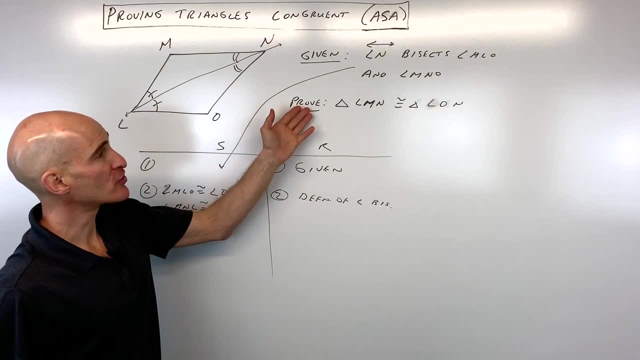 starting off, they like to just get the givens out of the way by writing them first. Whatever you're trying to prove, that's going to be your last statement. We're just trying to fill in the in-between statements. Okay, now it looks like we figured out everything that we can from the 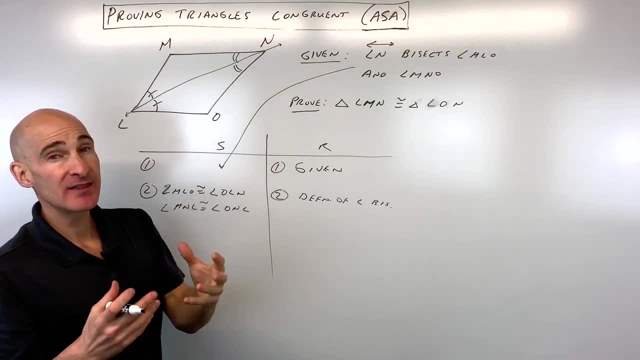 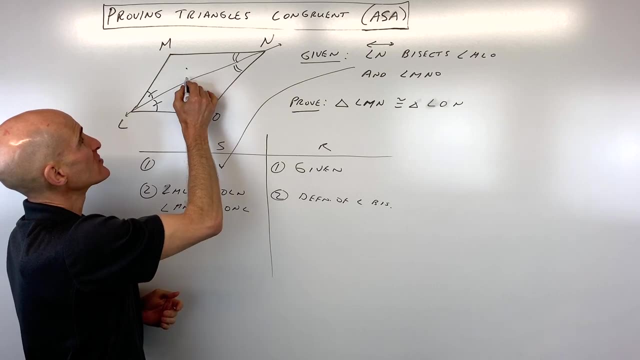 givens. Now I like to go to the diagram. I like to say: well, is there anything that I can show is congruent between these two triangles from the diagram? Well, it looks like they're sharing this side. These two triangles have side LN in common. So I'm going to say for step number three: 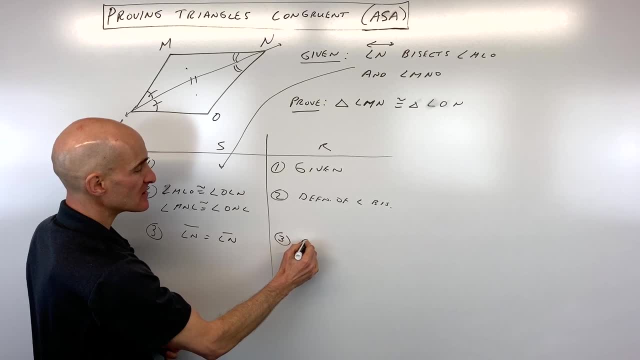 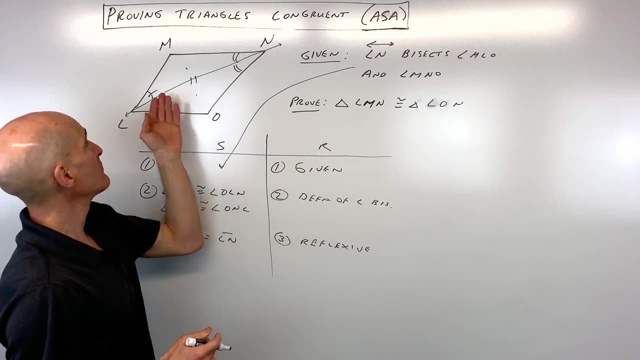 is congruent to LN, And the reason for that is the reflexive property. So it's just like looking in a mirror: You're the same height in the mirror as you are in real life, meaning that LN is going to be the same in both triangles. It's going to be congruent to itself. Now you can see that these 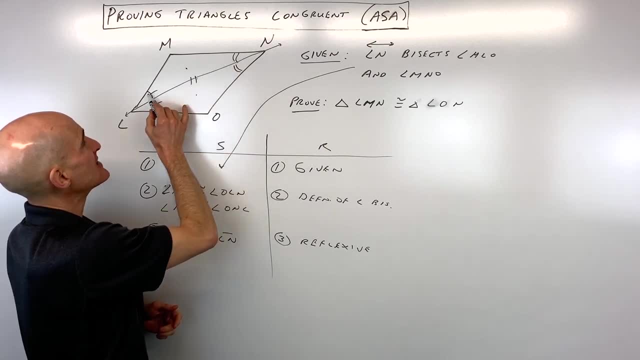 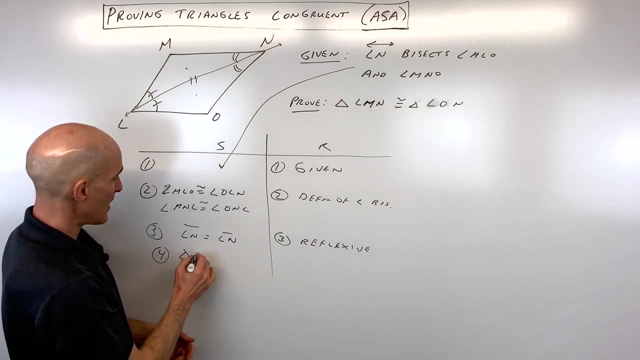 two triangles are congruent by angle side angle, The side is in between the two angles, That's what they call the included side. So that's going to be our last step, what we're trying to prove. So triangle LMN is congruent to LN. 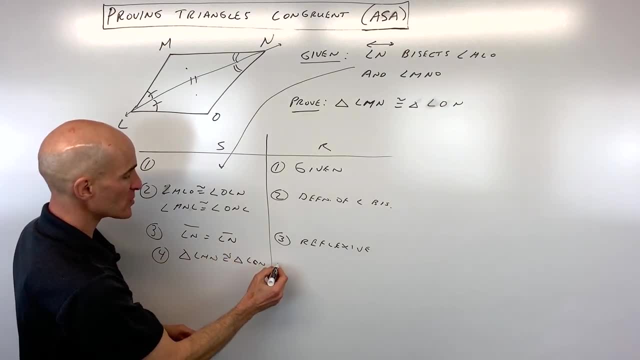 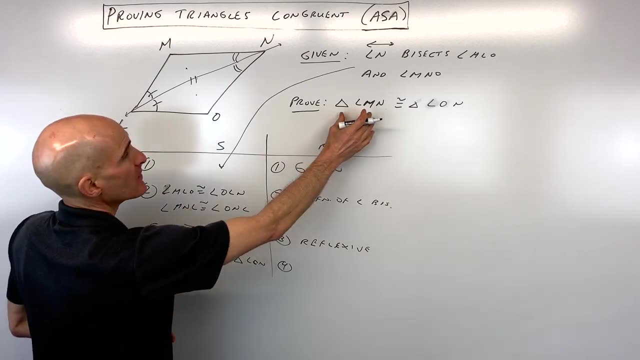 And again, you want to make sure that the corresponding vertices and the corresponding angles, the corresponding sides, et cetera, the ones that are congruent to each other, are going to match up. The order is important. So it looks like LMN is congruent to LON. You can see if you.